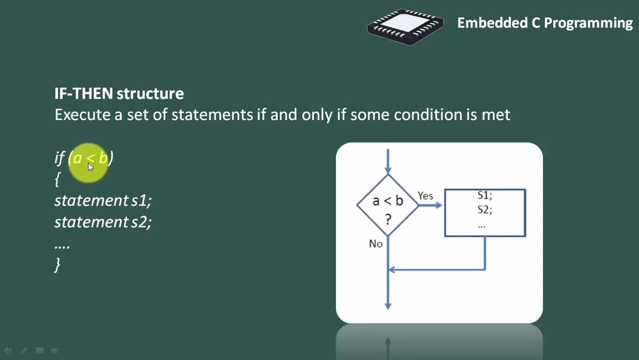 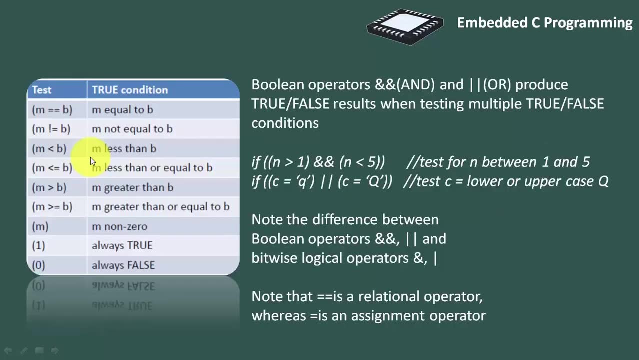 executed Here. for comparison, we have used less-than operator. In place of this less-than operator, we can use other operator like equal to 0.. We need equal to non-zero望장. therefore, בא familiar, 저희 passive avatar is not equal. 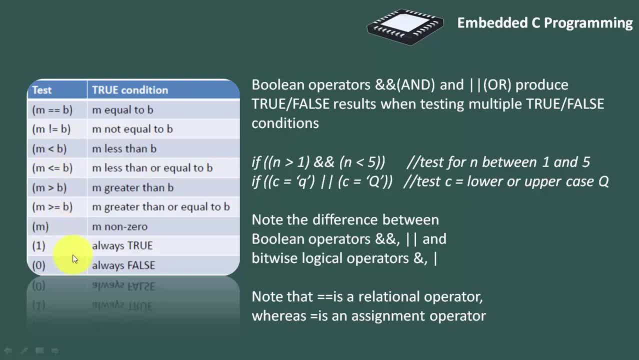 to less than 0 and non-zero是什麼 eligibility is equal to 0 and is less than or greater than 0. if we keep the non-zero value, like 0, than ix is not equal to greater than greater than equal to any non-zero value will consider as a true as 0 is considered as. 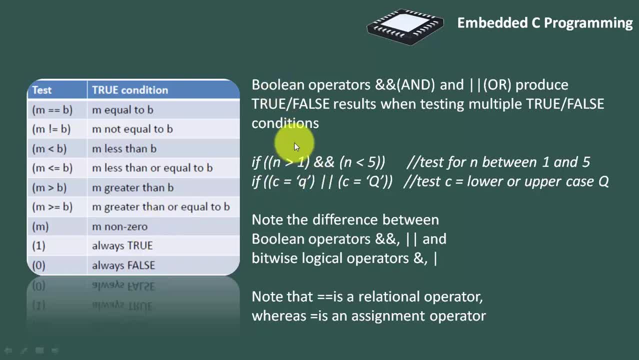 false. to combine one or more conditions. We can use Boolean operators. double amplace on is a AND operator and Boolean operator. We can use different classrooms likerand parameters, boolean operator. Here is the example: if n is greater than 1 and n is less than 5, when 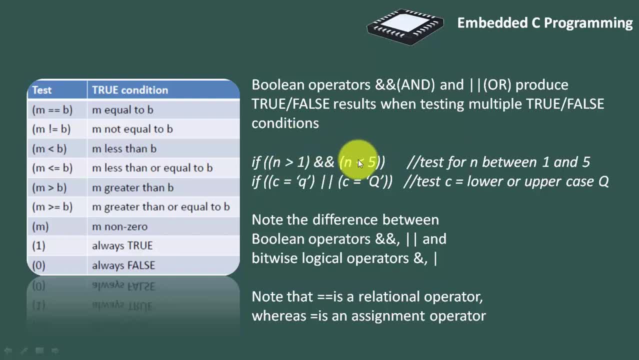 this, both condition become true, then only the entire condition become true. and if statement get executed in this example, if either of this condition is true, if statement will get executed. Please note that double ampersand and double vertical line are the boolean operators and not a bitwise operator. Bitwise operator. we will write like this: single and and single. 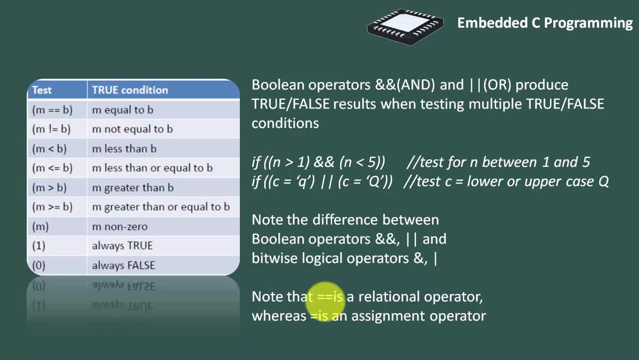 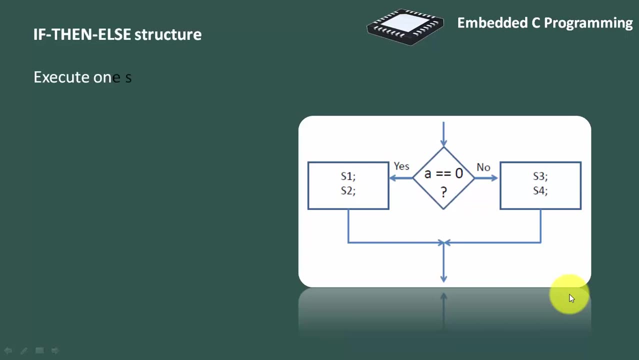 vertical line. Here also, you note that double equal to sign is a relational operator, whereas single equal to sign is the assignment operator. Okay, Now let's quickly look at: if, then else structure In. if, then else structure structure execute one set of statement if the condition is made and an alternate set if the condition is not. 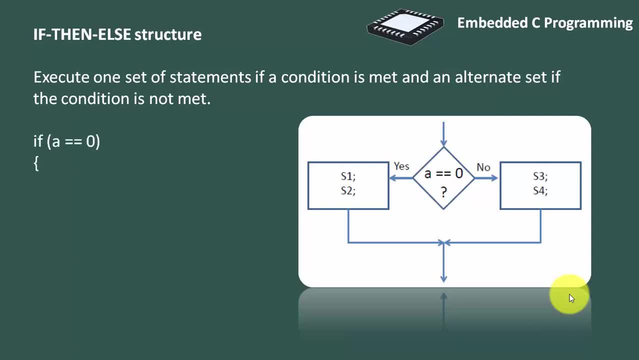 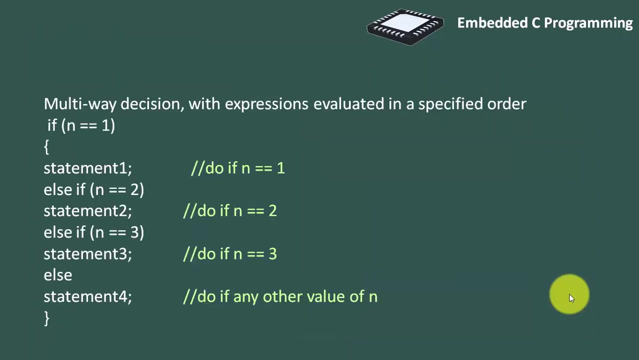 made. For example, if a equals to equals to 0, then the statement 1 and 2 will get executed. else the statement 3 and 4 will get executed. What if we want more condition to be tested? in that case you can use nested if else statement. For example: 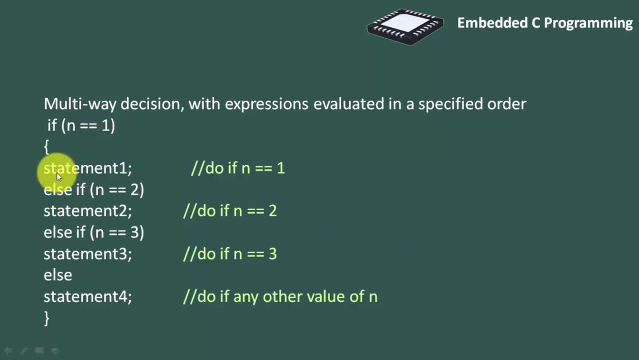 if n equals to 1, then statement 1 will get executed. else, if if n equals to 2, if this condition is true, then statement 2 get executed. if n equals to 3, then this statement is executed. if not 1, 2 or 3, then statement 4 will get executed. 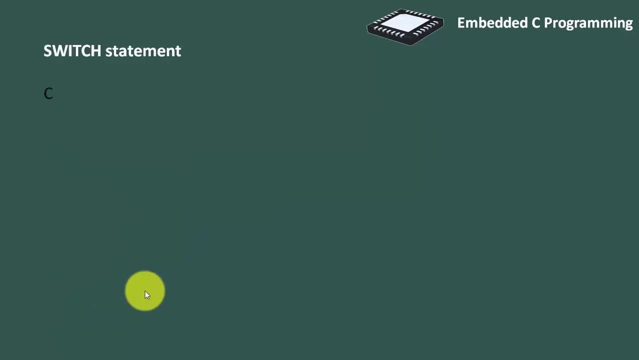 Switch statement. Switch statement is the compact alternative to else-if structure For multiway decisions that test one variable or expression for number of constant values. Here is the example: if the value of n is 0, statement 1 get executed if the value of n. 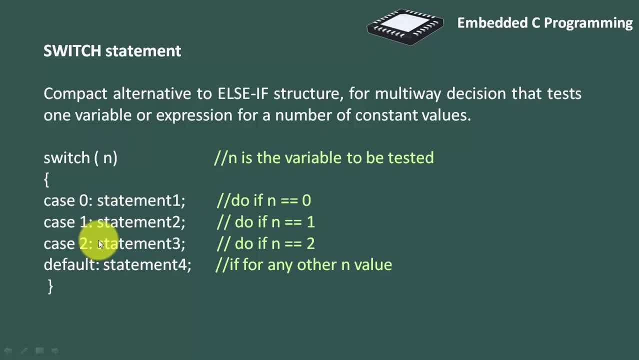 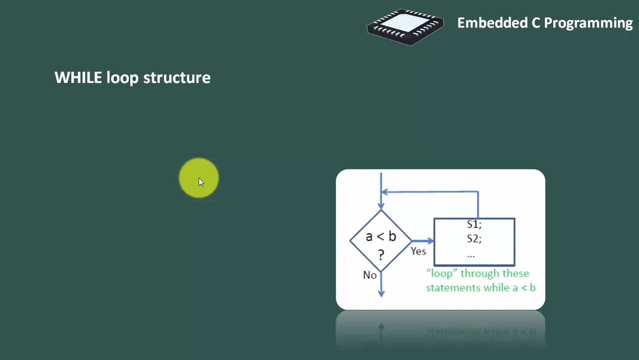 is 1, statement 2 value. if the value of n is 2, then statement 3. else, if the value of n is 1, statement 2 value. if the value of n is 2, then statement 3, else, this, by default, is statement for fill: get executed. Now let's see iterative C control structures. 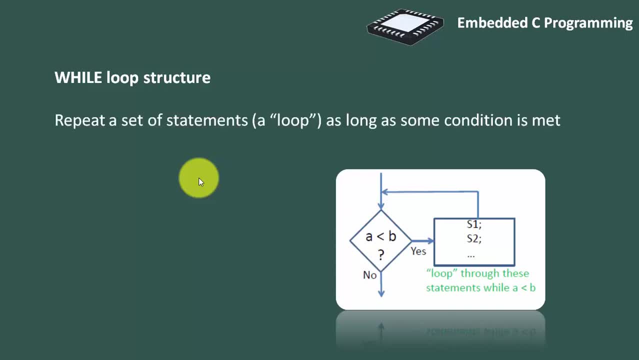 First one is while loop structure. Here we repeat a set of statements as long as some condition is met, For example, while a is less than b. Till the time this condition is true, statement 1 and 2 will get executed continuously, since it is in a loop. When this 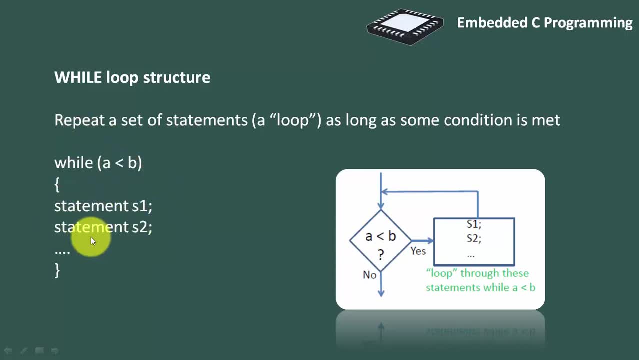 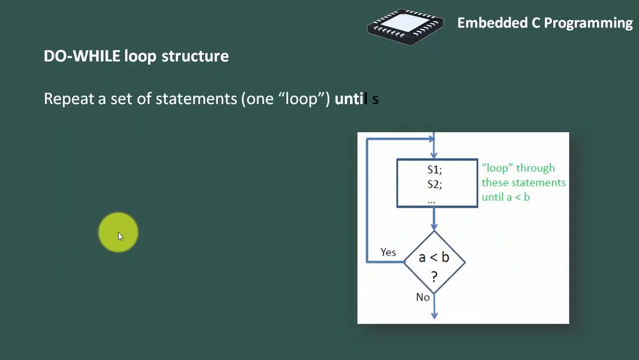 condition will become false. the while loop will get terminated. Do while loop structure: Here we repeat a set of statements until some condition is met. Here is the example You can see here while condition is tested after do statement, since the condition is. 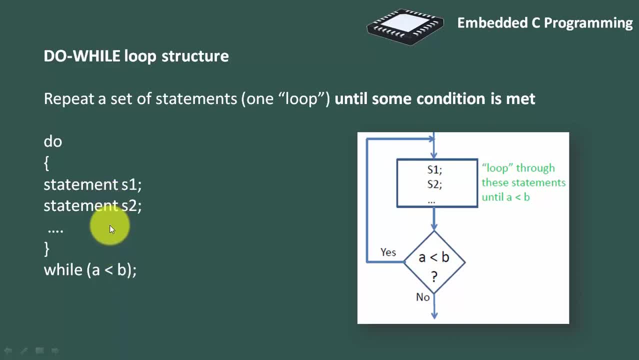 tested after the execution of set of statements. so the statements are guaranteed to be executed at least once. So first statement 1 and 2 will get executed and then we will check for while condition. Now, if this condition is true, then again statement 1 and 2 will get. 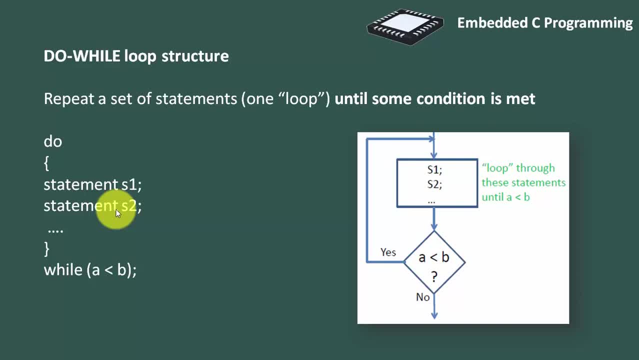 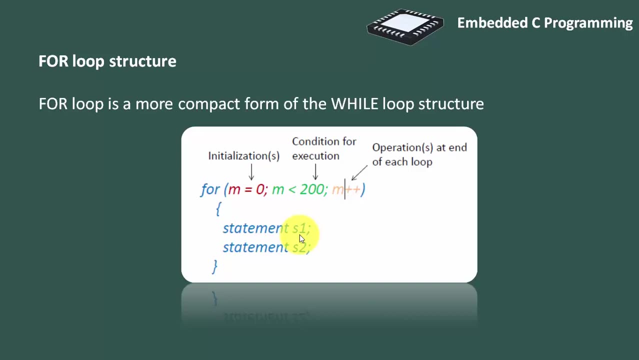 executed. Do while loop guaranteed that the statement 1 and 2 will get executed at least once, since the while condition is getting checked after. do statement For loop structure. For loop is a more compact form of while loop structure. Here is the example: For m equals to 0, m is less than 200, m++. This condition is what we call initialization. 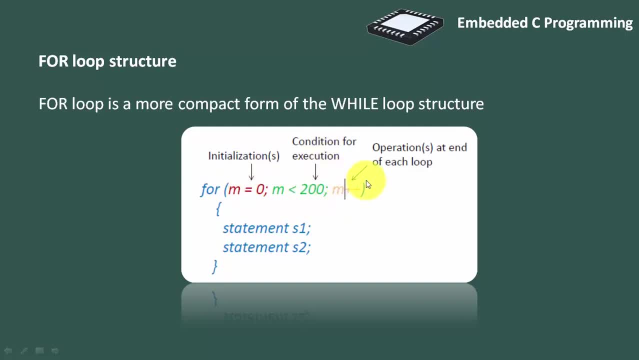 This is what we call initialization. This is the condition for execution, and this one is operation at the end of each loop. Initially, the value of m is 0. Since value of m is less than 200, the statement 1 and 2 will get executed, and then the value in m will get incremented by 1.. So this loop will 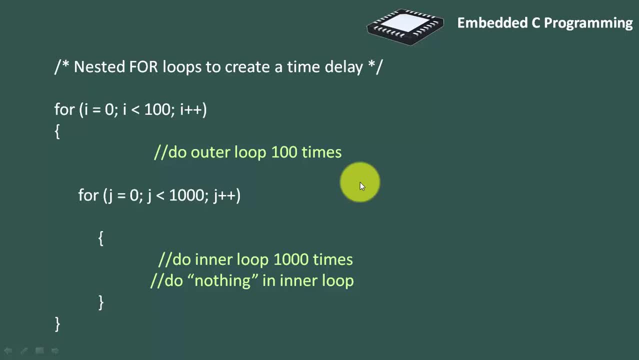